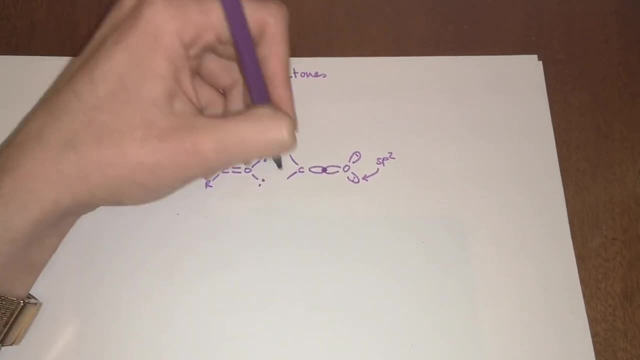 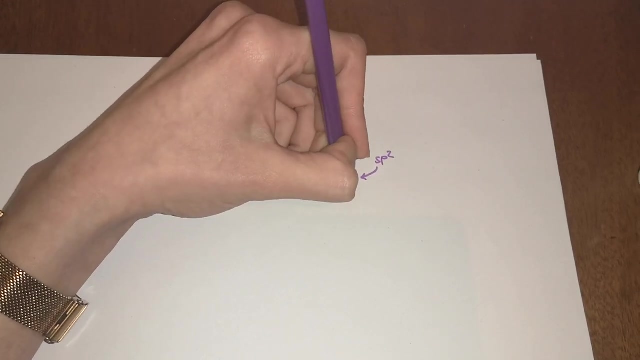 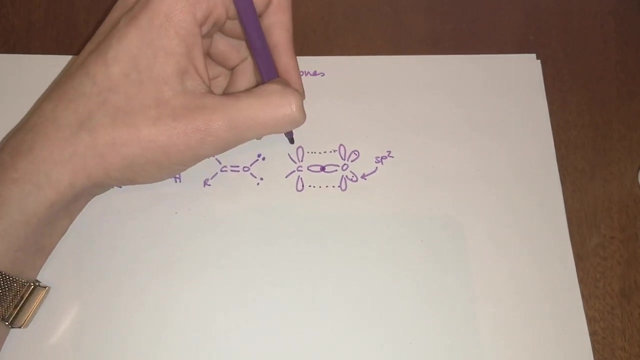 and then what you have. so then you have your two other bonds on that carbon, and then you have your two p orbitals which stick up and down, above and below the molecule, and then again, despite looking really far away, these overlap to form your side on overlap, your pi bond. Okay, so similar to alkenes. 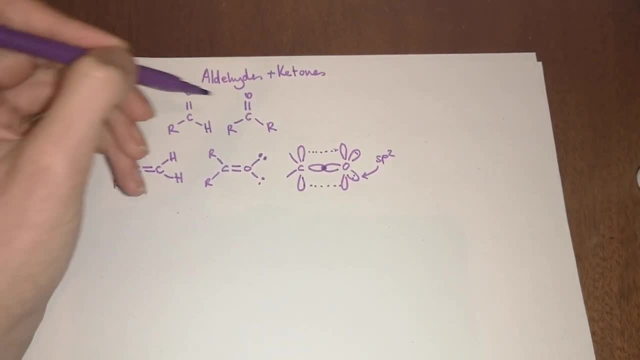 a carbonyl doesn't rotate. however, in terms of what the molecular orbitals look like, in this case it doesn't really matter, because of the fact that you've only just got lone pairs. you haven't got substitution at all. Okay, so just to bear in mind that it doesn't actually rotate. 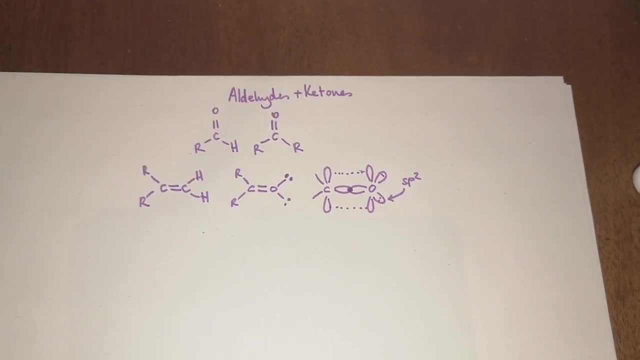 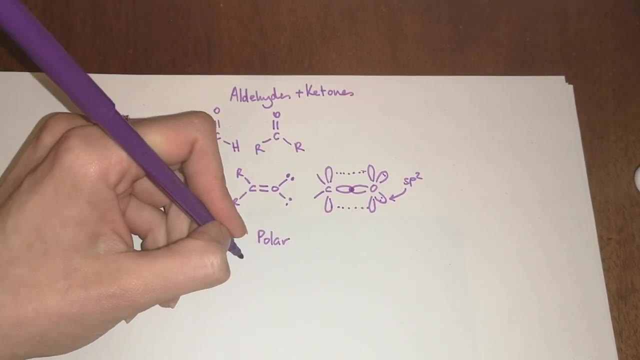 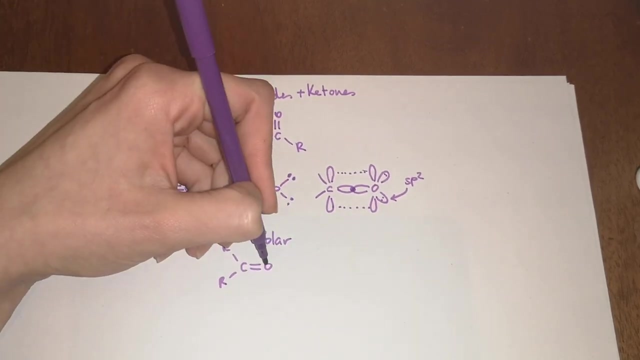 Other properties of aldehydes and ketones and other carbonyl containing molecules that are exceptionally important is that they are polar. Okay, so, as I've said before, if you have your functional group, whether it be an aldehyde or a ketone, your oxygen is more electronegative, so it's. 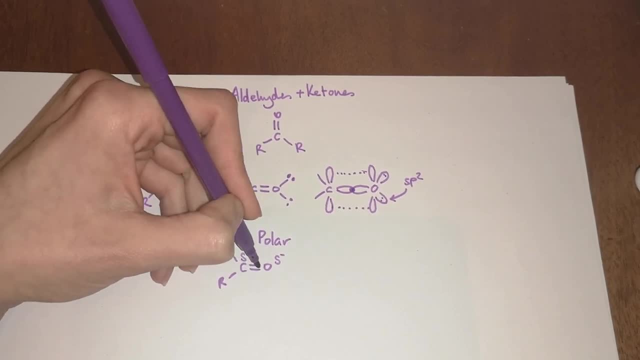 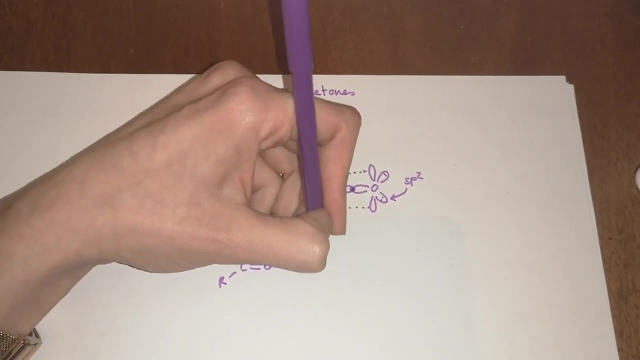 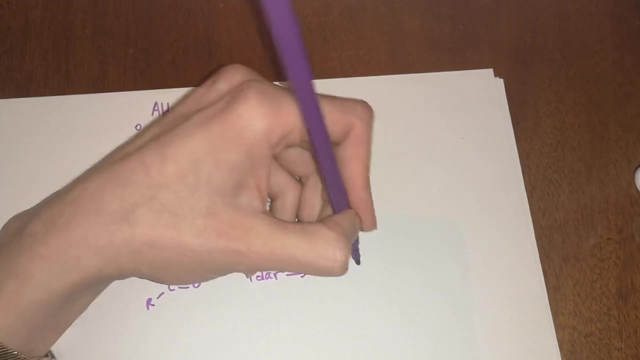 positively charged and your carbon is slightly positively charged, and that's because the two pairs of electrons in this carbon-oxygen double bond are pulled towards the oxygen. Okay, so that means it's polar Okay, and what that also means is that small ones, so small molecular weight. 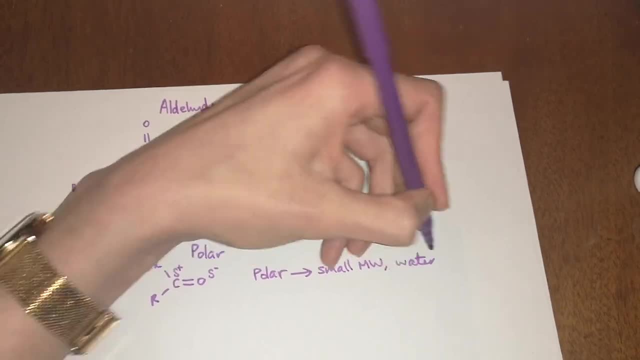 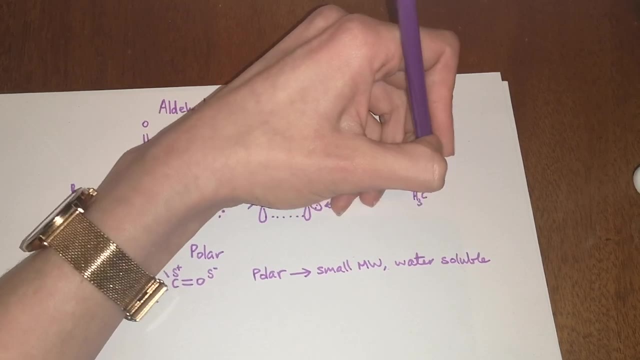 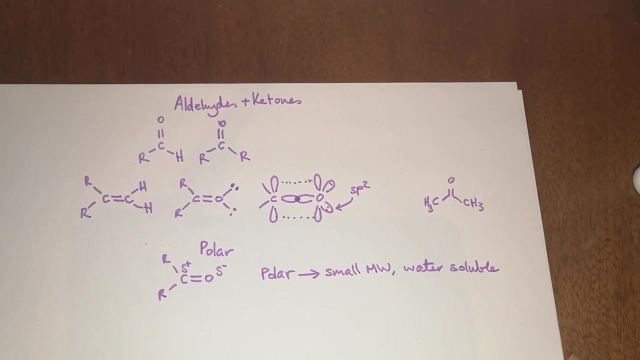 compounds are water soluble, Okay, so an example of that would be acetone. Okay, so it's usually used as nail polish remover, or if you've got particularly sensitive skin, you might use an ester instead, but this is soluble in water. so if you mix acetone or nail polish, 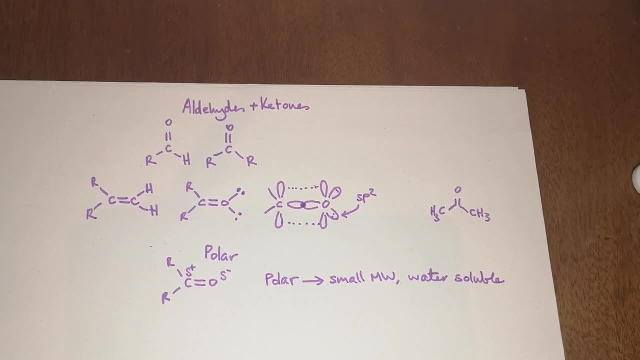 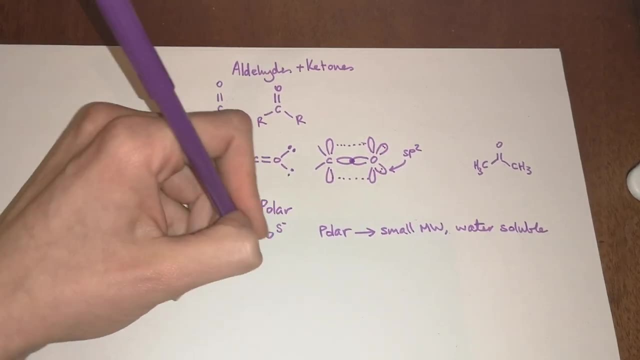 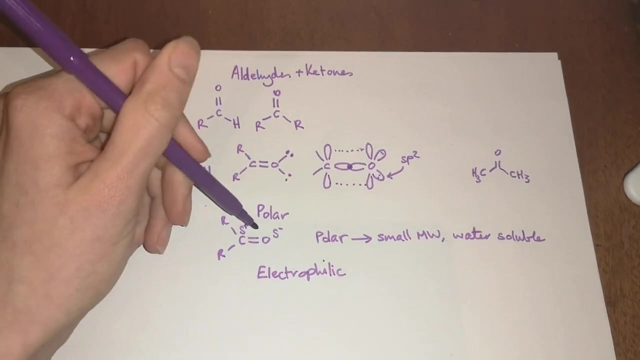 remover or water, you'll just get one big solution. You won't have two layers in your glass, Okay, another really important part of the fact that it's polar is that it is electrophilic. So, as we said before, even though oxygen has, 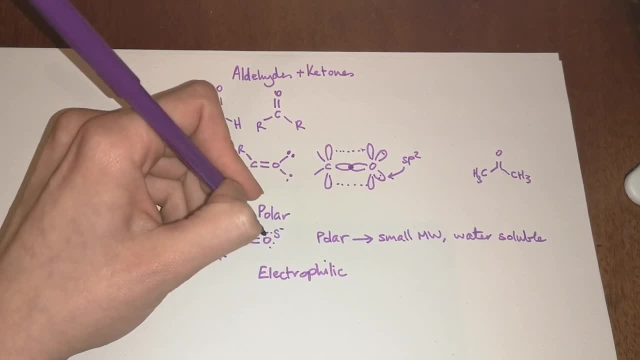 two lone pairs. it's very electronegative so it doesn't like to donate those lone pairs to form another bond. So this is not nucleophilic, Even though you have negative charges, the oxygen, apart from very special cases and different types of functional groups where you have ketones and you've 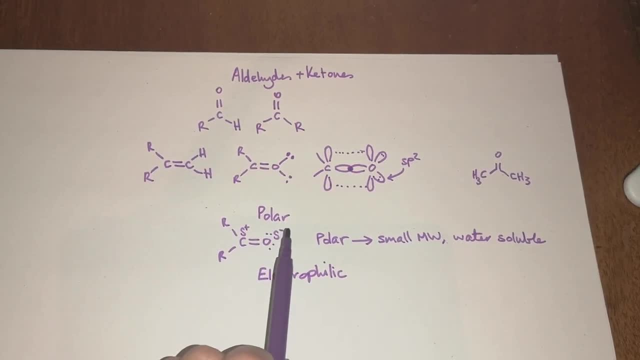 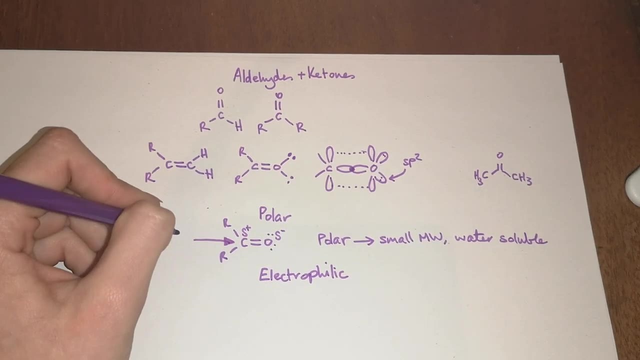 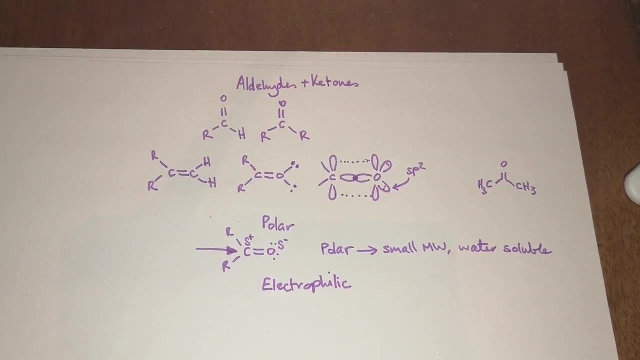 got other ore groups here. this oxygen generally does not do any attacking ever. Okay, what happens is it's electrophilic at the carbon. Okay, so that means nucleophiles, things that have lone pairs or negative charges or a pi bond. They can attack this carbon. Okay, so the general mechanism for that would be whether you have an 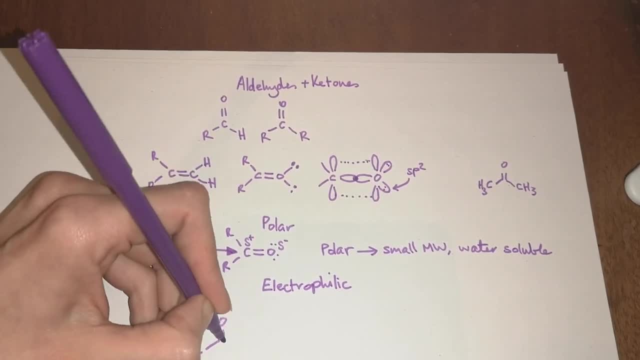 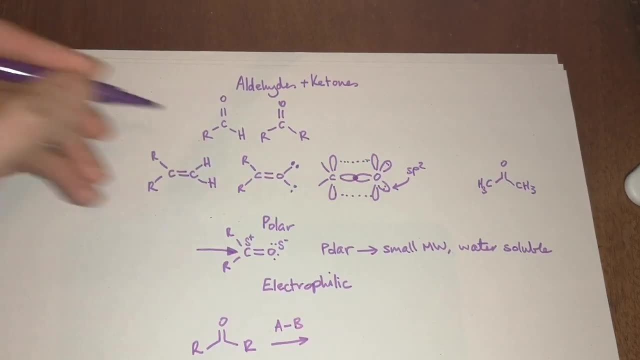 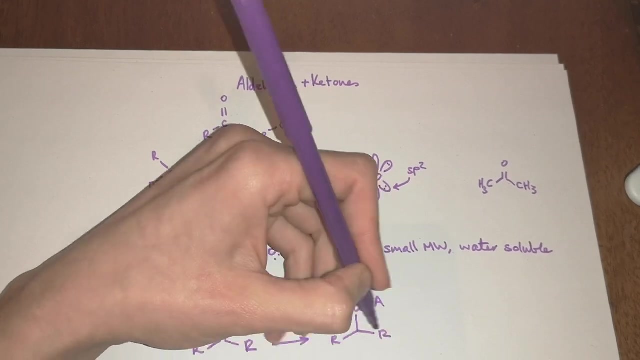 aldehyde or ketone, it doesn't really make too much of a difference. Okay, you would have molecule A, B, Okay, so it doesn't really matter what it is. what will happen is A will add to your oxygen after B adds to the carbon. Okay, so 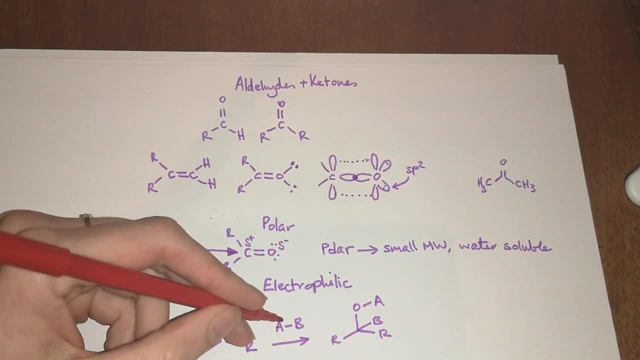 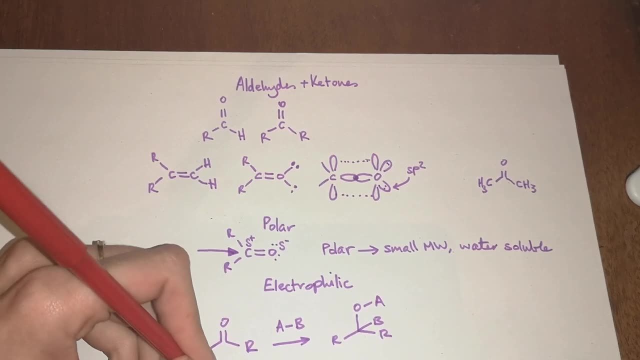 in terms of the mechanism. what that would mean is, for example, if you had some nucleophile, Okay, so let's say B is your nucleophile. Actually, you know what? just to be clear, we're going to say NU minus Okay. so whichever part of this AB molecule is nucleophilic, that's going to attack your carbon, So it has a negative charge. 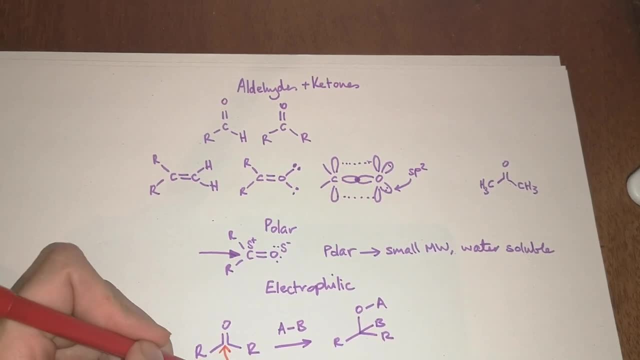 and it attacks the carbon. So remember the way the arrows are drawn: they start at the, where the electrons are, and they finish right on the carbon that you're attacking. But carbon cannot have five bonds, So it has one, two, three, four bonds at the moment. So you have to break an old 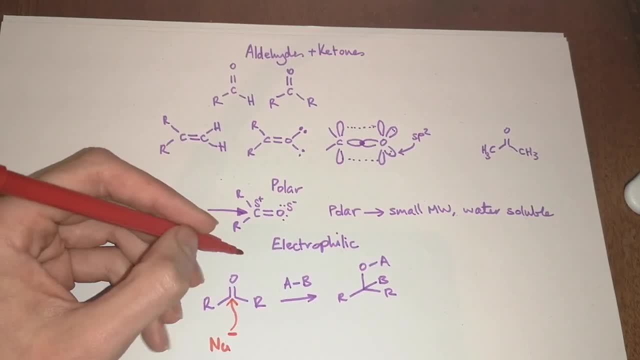 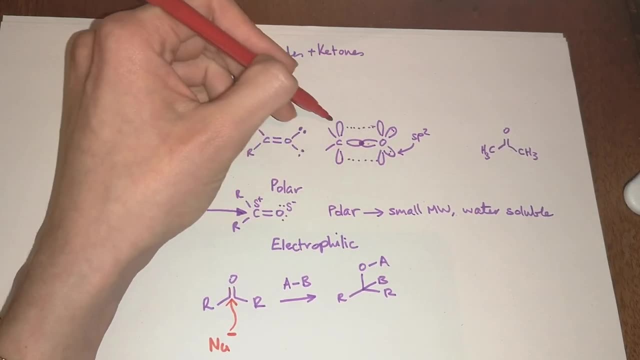 bond. Oh sorry, I pushed that up. So you're going to break the weakest bond. and because sigma bonds are head-on overlaps, they're quite strong, But pi bonds are only side-on overlaps, so they're quite weak. So you're going to break the double bond and the electrons are going to end up back on the 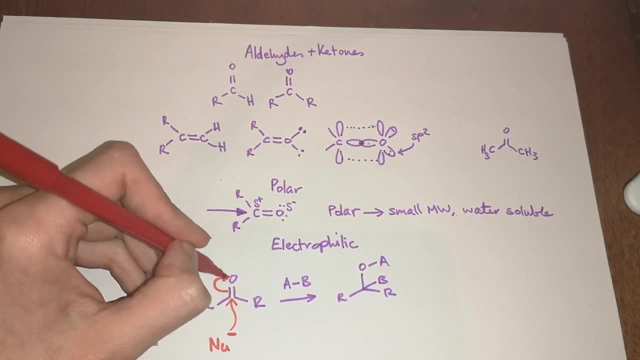 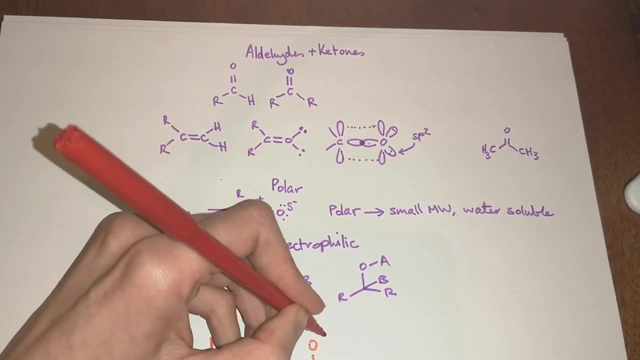 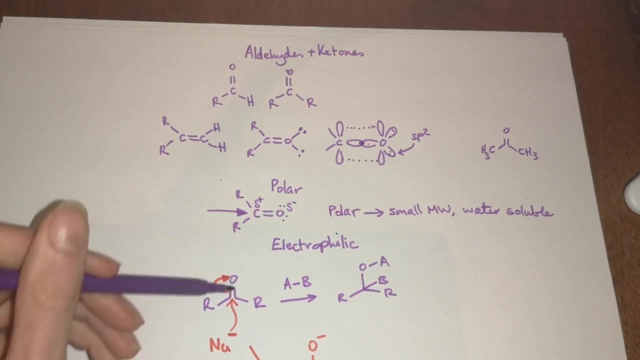 oxygen. And it's really important again to show: the electrons came from the dual bond and they end up on the oxygen. So then what you end up with Is this molecule here. Okay, and again, it's really important to remember that when we started on in this side, there was 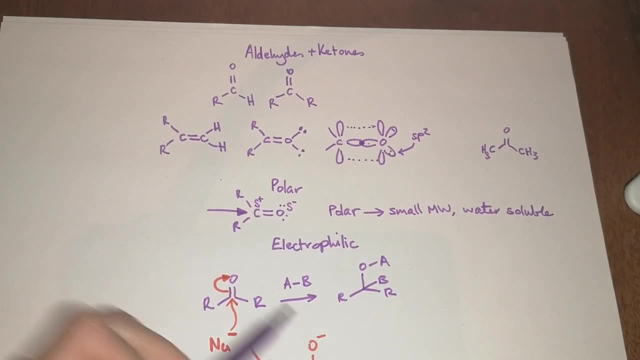 one negative charge. So you have to remember to put a negative charge on your oxygen, because before it used to share two electrons with the carbon, But now it has both of those electrons to itself and that's why it has a negative charge. Okay, so then the next thing that will happen: 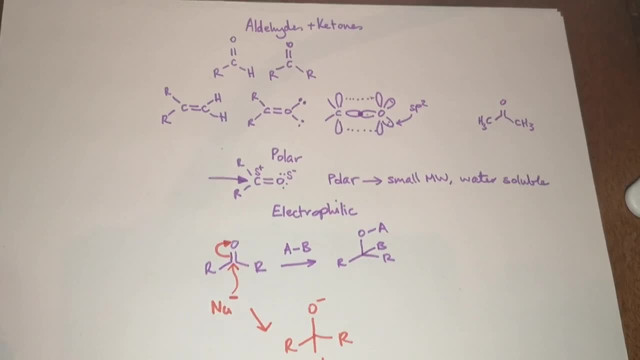 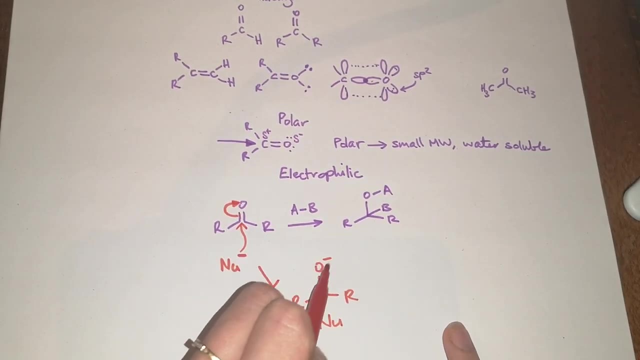 usually after you do the reaction, what you'll do is Have I- Yes, I keep on leaving the page down too low, Sorry about that. So, after the nucleophile attacks, you break the double bond and you end up with a negative charge in the oxygen. So then, usually after you do a reaction like this, what you'll do is you'll 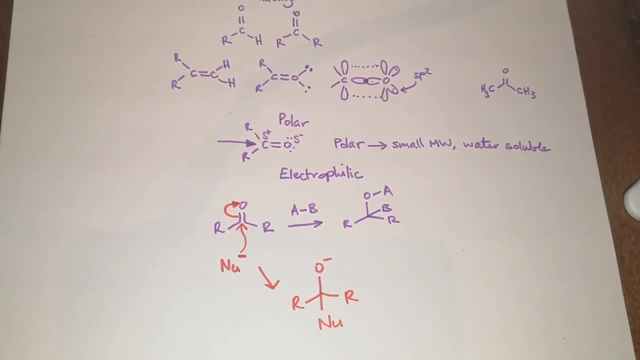 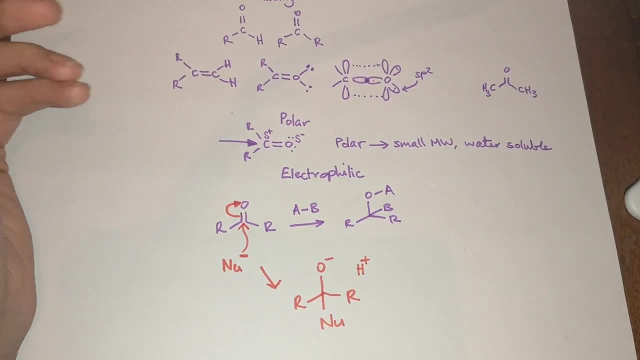 actually mix. whatever your reaction mixture is, whatever the solvent is, you'll mix it up with maybe a little bit of acid and water, So you'll have H plus. you'll have protons floating around next to your alkoxide and the negative charge of the oxygen will attack the hydrogen. 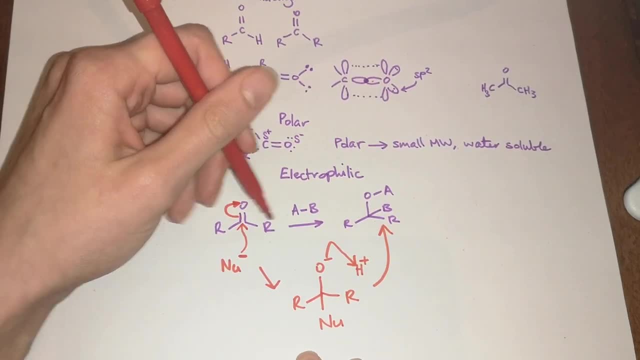 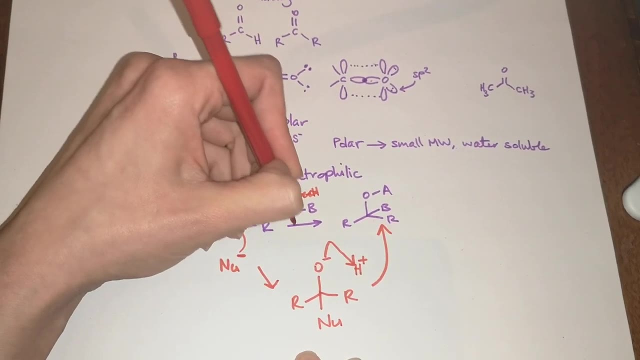 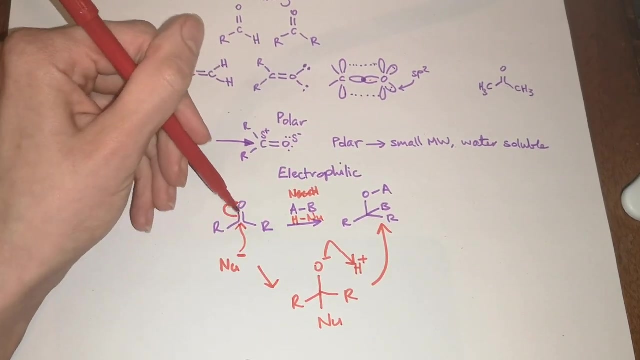 So then, what you'll end up with is this. So, overall, what you've done is: so, if this was, AB is equal to NUH. Okay, actually I'll draw that the other way around: H and U, just so it matches what I've drawn here. Okay, overall, you're adding something to both of the atoms in the carbonyl. 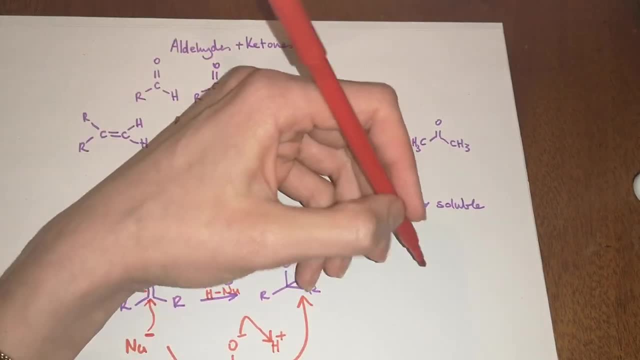 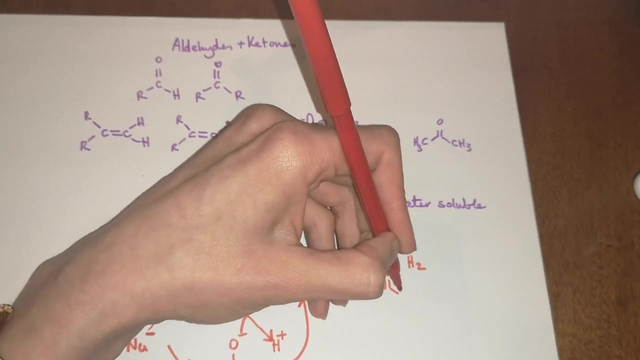 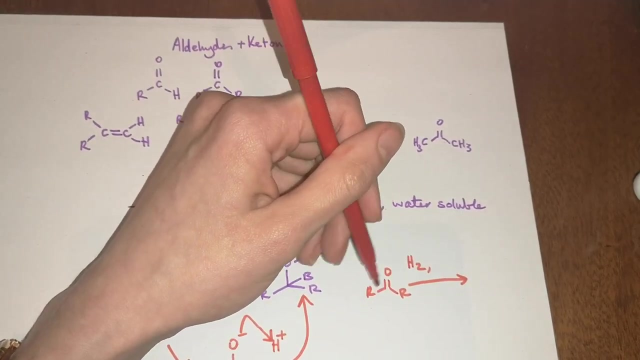 Okay now, the most common example of that, possibly, is the addition of H2.. Okay, so if you have either a ketone and you add hydrogen gas and again, as we've seen with the alkenes, hydrogen doesn't really want to add one atom at a time, So you're going to use a catalyst like nickel or palladium. 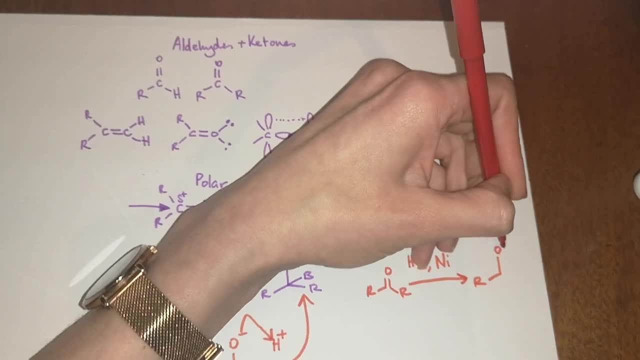 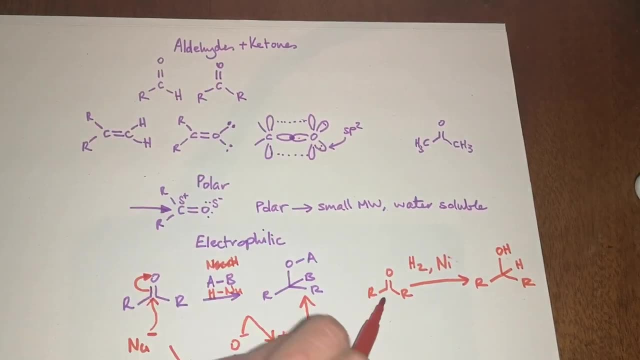 Okay, and what will happen is you'll add one hydrogen to the oxygen and you'll add one hydrogen to the carbon. Okay, so when you do it with the ketone, you end up with a secondary alcohol. So this carbon has two ore groups on it, so this is a secondary. 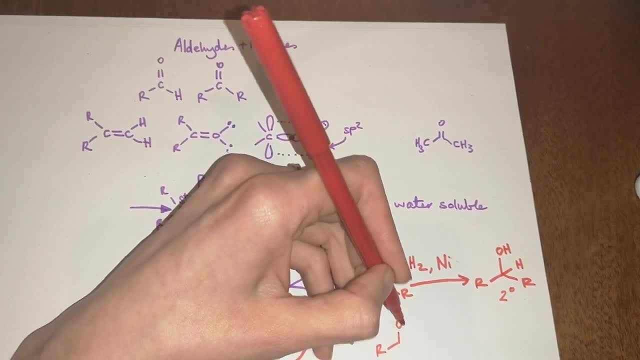 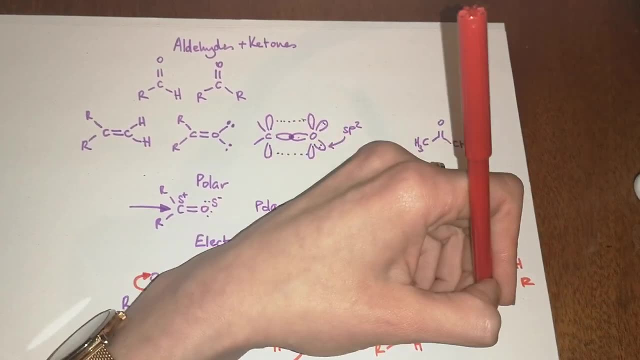 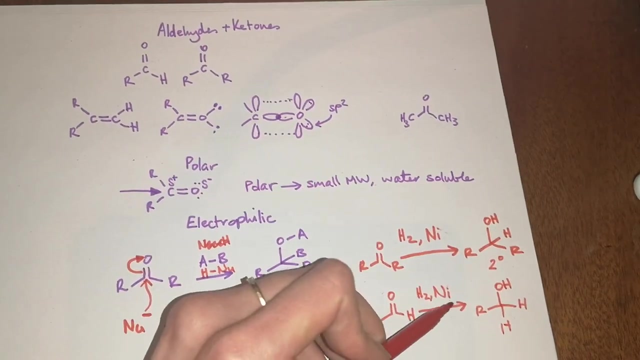 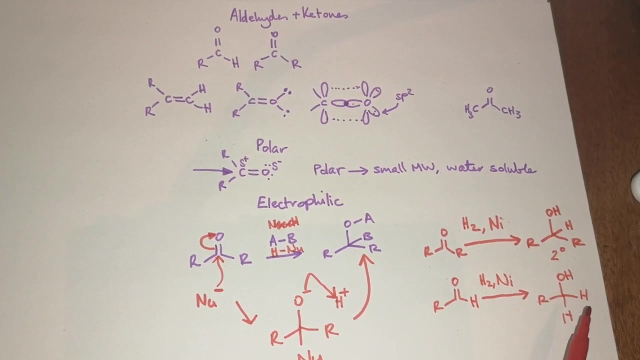 Whereas when you do this to an aldehyde, using the same conditions, so H2 and nickel- you end up with a primary alcohol. Okay, because there's only one ore group attached to the carbon of your hydroxy group. Okay, so this is known as a reduction. Okay, so the next video is actually 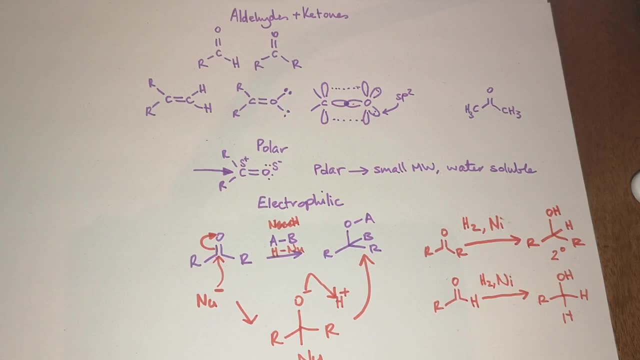 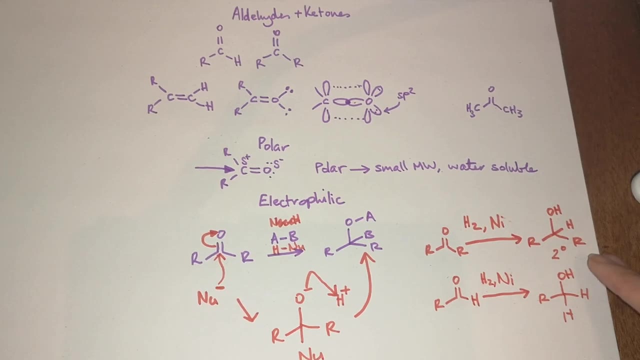 going to be just on oxidation and reduction. How do you go from alcohols to ketones or ketones down to alcohols? How do you get carboxylic acids and etc. And it's a really, really important thing in organic chemistry being able to move through oxidation. 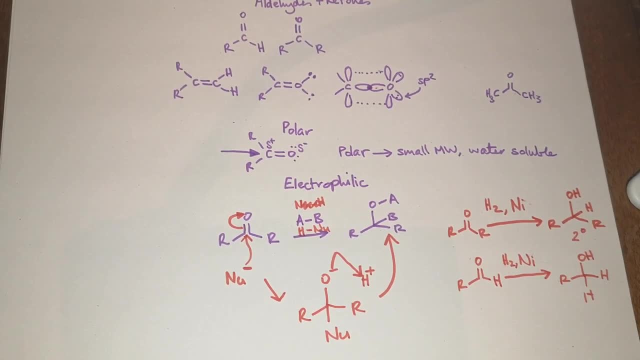 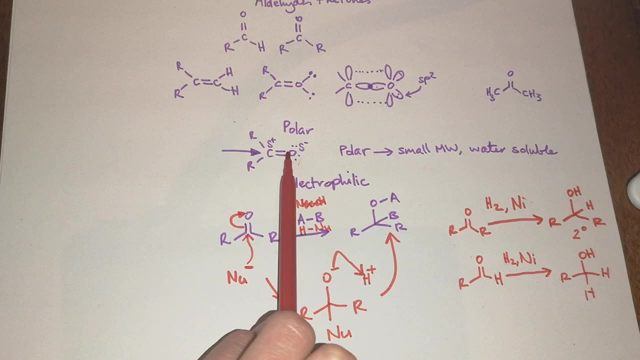 states. So that's really all you need to know about aldehydes and ketones. Okay, so because they're polar, they can accept hydrogen bonds, but because they don't have an OH themselves, they cannot donate hydrogen bonds. So this means they have lower boiling points than alcohols. 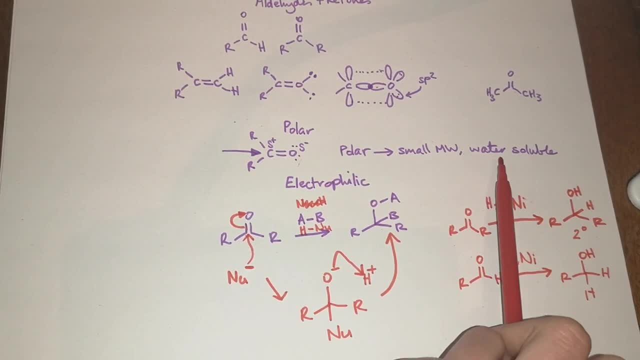 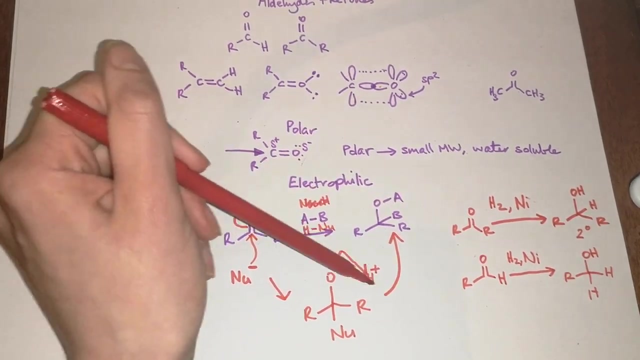 Because they're polar, if they're water soluble and the most common reactions that ketones and aldehydes undergo are nucleophilic attack. Okay, so the carbon gets attacked by a nucleophile, You break your double bond and then your oxygen, most commonly, will pick up something like a proton. Okay, so, if you found this video, 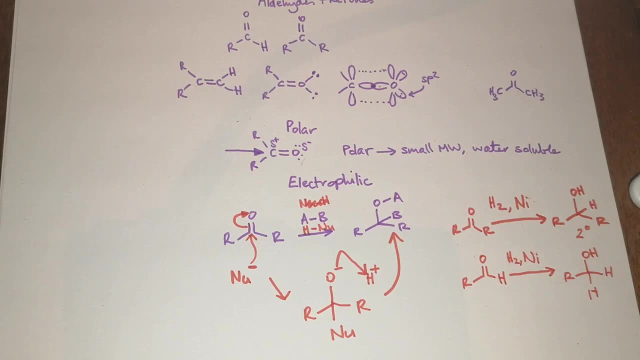 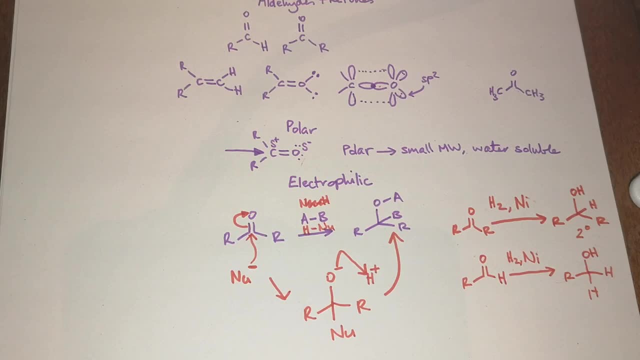 donations, the more videos that I am going to try and make before your exam on the 13th of November. So please do check that out and I will see you next time. 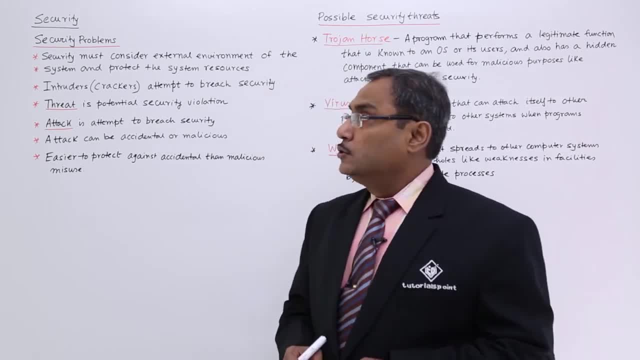 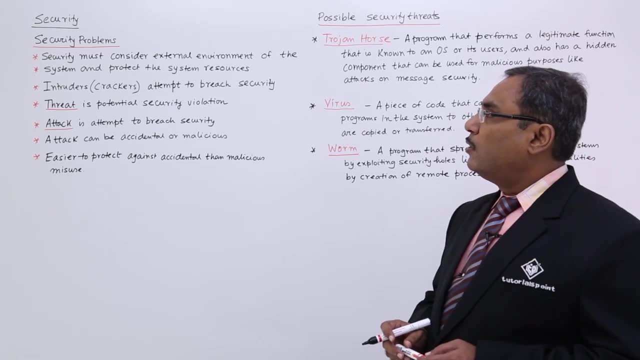 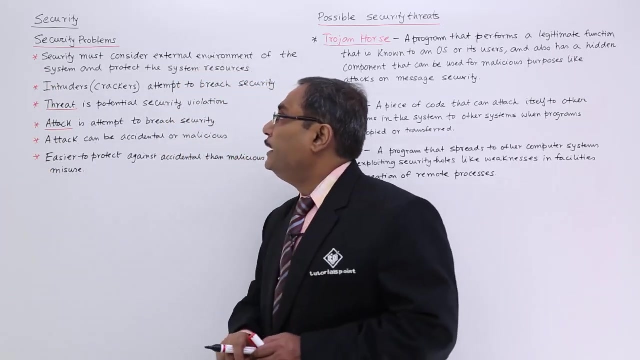 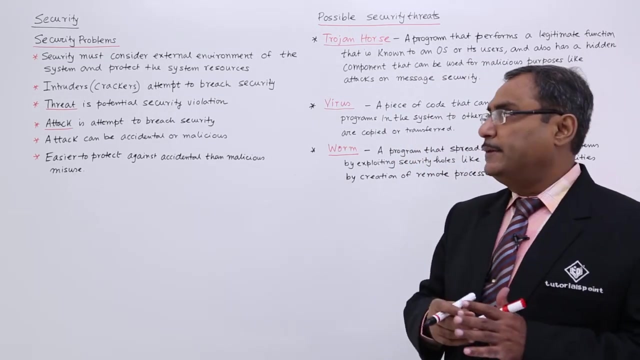 More on security in this particular session. So let me tell you what are the security problems. Security must consider external environment of the system and protect the system resources. So that means in case of security, it must consider the external environment. That means the different users. they will be coming from outside to the particular system. 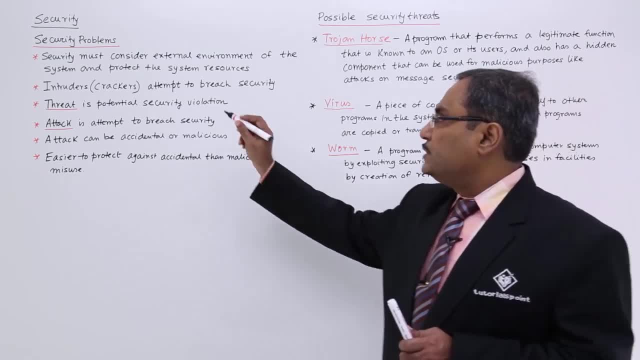 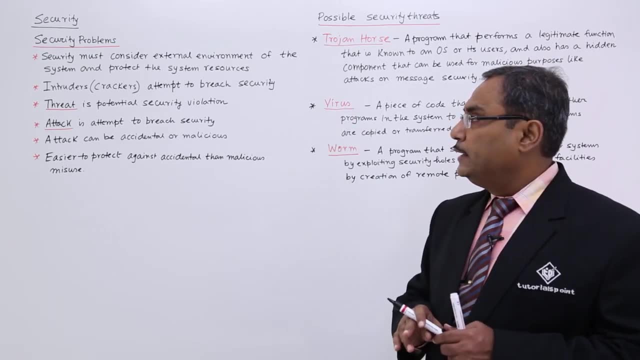 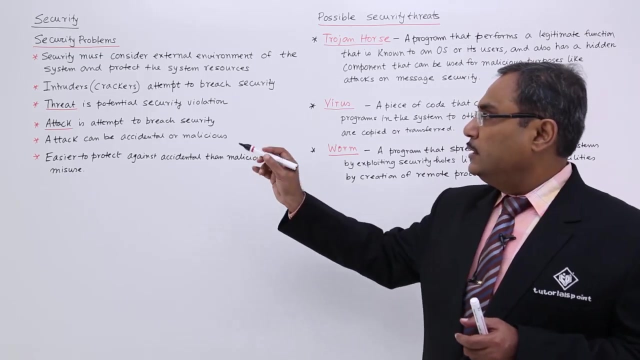 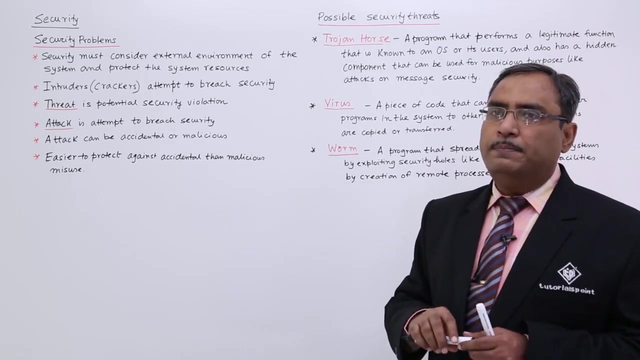 and how to protect the system resources, how to protect the system resources from those from those external environment. that is a main security problem. Intruders can also be called as crackers. Intruders means trespassers, rather unauthorized persons. they will always try to attempt to breach the security, So obviously that is the main purpose for that.